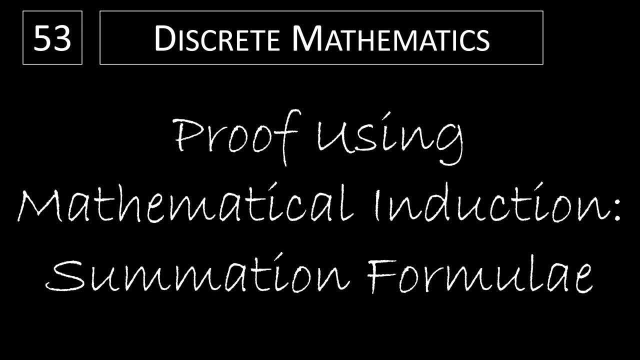 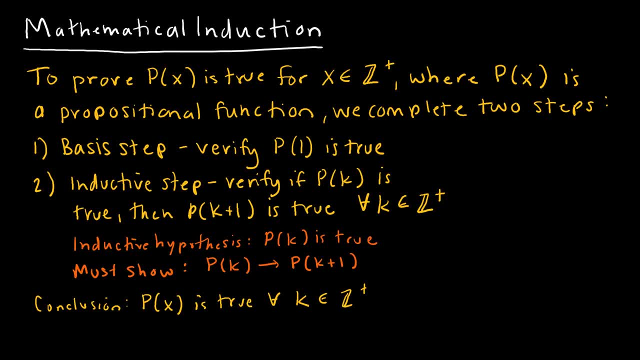 In this video, we're going to take a look at solving linear congruences using the inverse. Before we do a proof with mathematical induction, let's talk about what the process is for mathematical induction. Mathematical induction is like a ladder with an infinite number of rungs and the thought process here is: 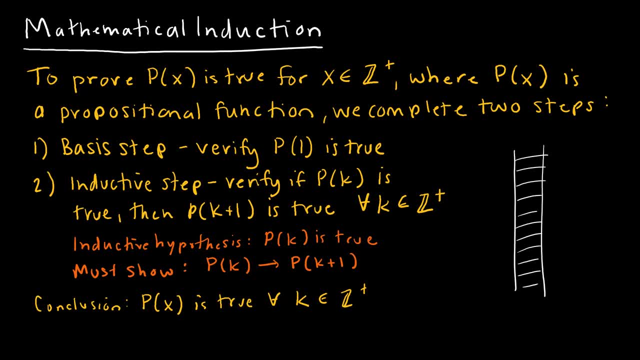 that if I can prove that I can get to the first step of my ladder, and then I can prove that if I can get to the first step of my ladder, if I can get to any rung of the ladder, including the first, then I can get to the next rung and then 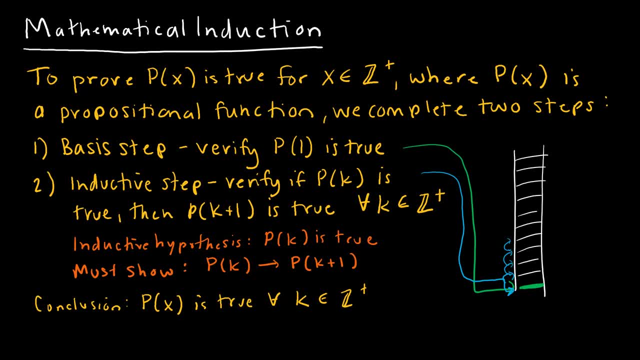 that tells me I can get to the next rung, and that to the next rung, and that to the next rung. then I can get to any rung of the ladder that I want, and it's true for all rungs of the ladder. 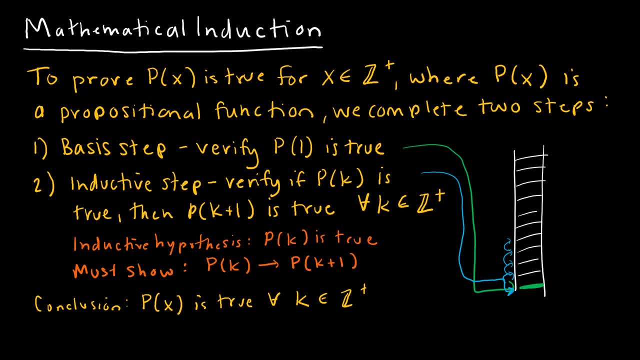 So what does that mean in terms of what we're going to do mathematically? Well, we're first going to prove a basis step, and the basis step says: I can get to the first rung of my ladder. I can verify that my propositional function p of x is. 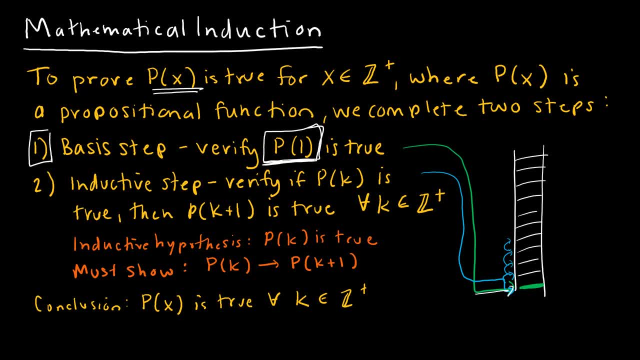 true for whatever my first value is. Now notice I have written p of 1, but it's very possible, depending on your situation, that maybe your first value that you need to prove is the value of the first rung of the ladder. So if I 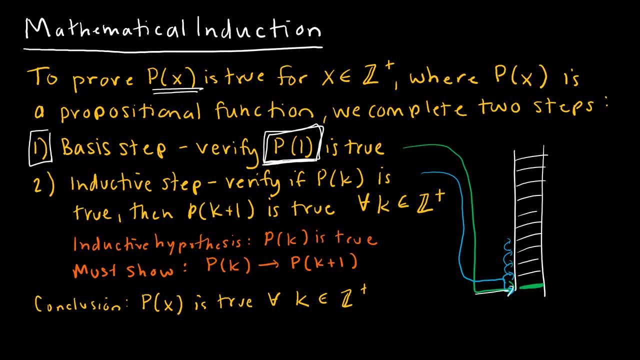 need to prove that my first rung of the ladder there is the first swoje that I can verify that it's true for 3 of the ladder. So then p of 3 would be your basis step From there. we have to verify that if p is true, then that implies 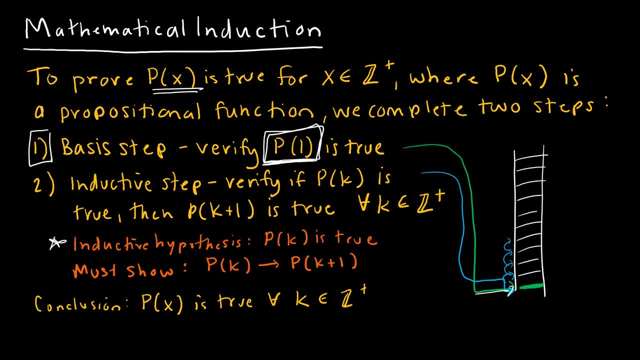 that p is true. So there's two parts that you're going to see me write and any video that you watch you should see any instructor write the inductive hypothesis. the inductive hypothesis says we're going to assume p is true. 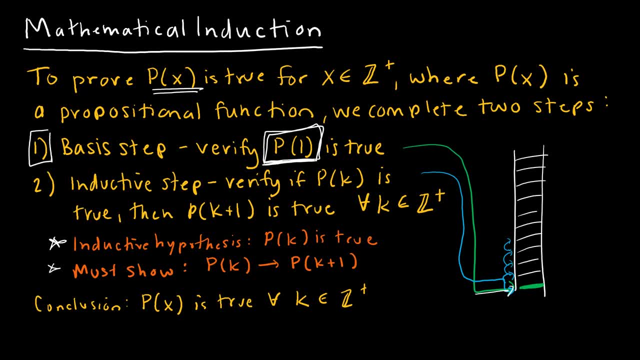 You will also see me write must show, and so a lot of instructors don't write what you must show. and then at the end they say: here, this is true, because I showed this. I like to be very explicit about it. I like to say: here's what I'm assuming is true. 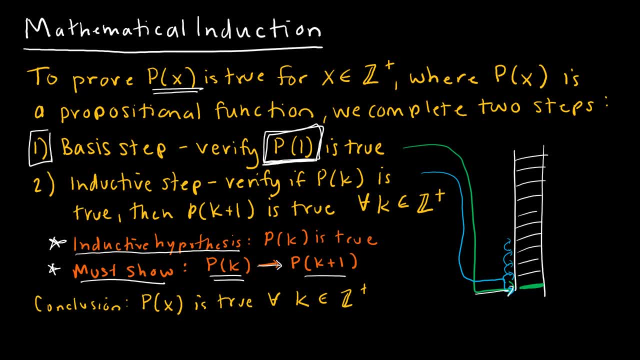 Because that's true. does that imply that P of K plus 1 is true? And if it's true that P of K implies P of K plus 1, and I can get to the first rung of my ladder, then I can get to every rung of my ladder. 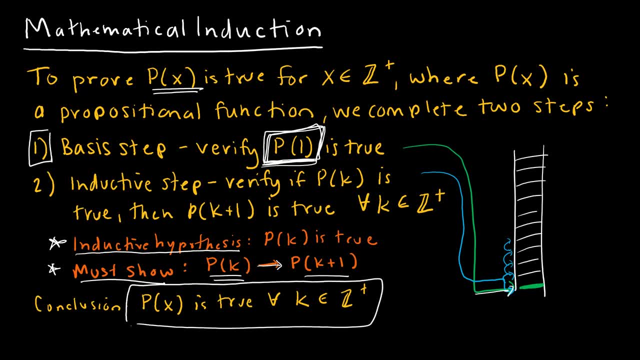 So my conclusion will be that whatever it is I'm trying to prove is true for all K that are positive integers. So let's take a look at our first example For our first proof: by induction we're going to prove a summation formula that we've already used. 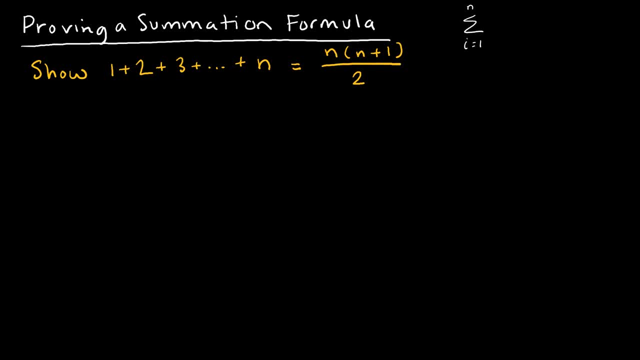 In this course, which is the summation as i goes from 1 to n of i, is equal to n times n plus 1 divided by 2.. So, as you can see, that's exactly what I have here, but on the left side instead of the summation. 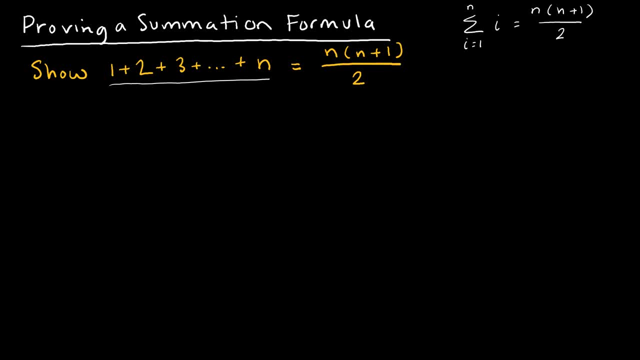 I've just written out the sequence of terms instead, And you'll see why in a little bit. When I start a proof by induction, I have to specify what it is that I'm trying to prove. So I have to tell what that P of n is equal to. 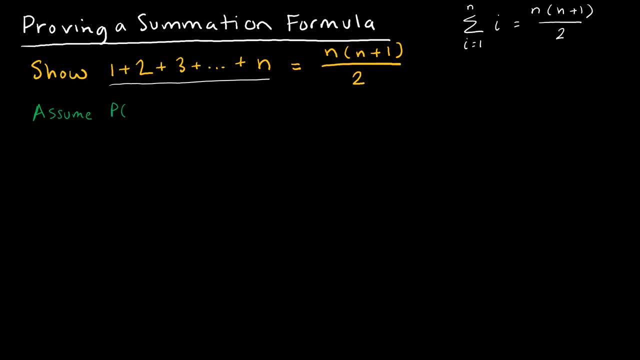 So I'm going to assume P of n, or let not assume. I'm just going to let P of n represent 1 plus 2 plus 3, all the way through. n is equal to n times n plus 1 divided by 2.. 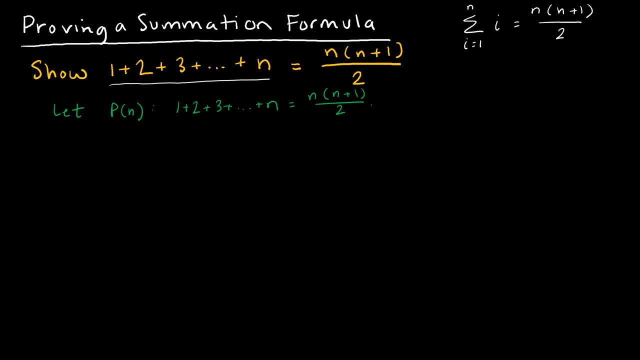 It's important that I do that step because that's saying here's what I'm trying to prove. So make sure that you are explicit about that step. Then I'm going to do my basis step. And the basis step, if you'll recall, says: prove P of 1 is true. 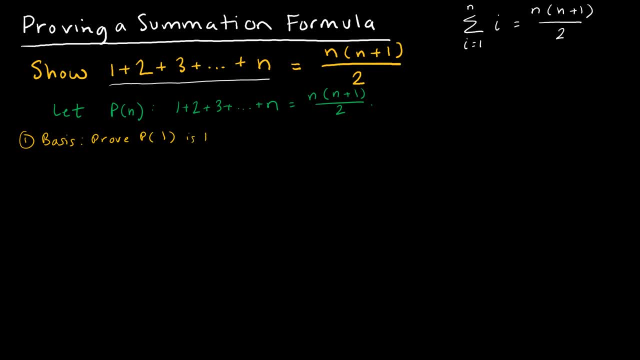 Prove I can get to the first rung of the ladder. Now, in this case, P of 1 would actually be 1, right? We're actually trying to prove that I can use 1 and find the solution. So P of 1.. 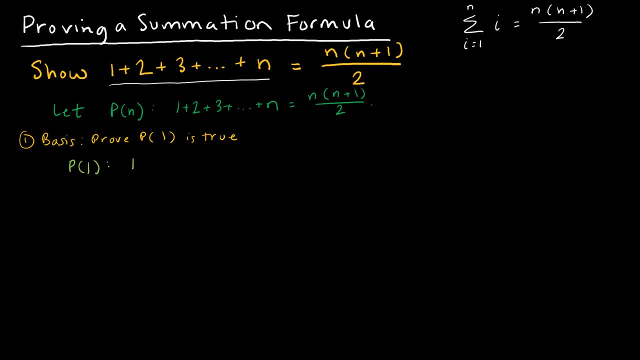 P of 1 would be: 1 equals 1 times 1 plus 1 over 2.. And I have to just verify that's true. On the left side, I have 1.. On the right side, I have 1 times 2 over 2.. 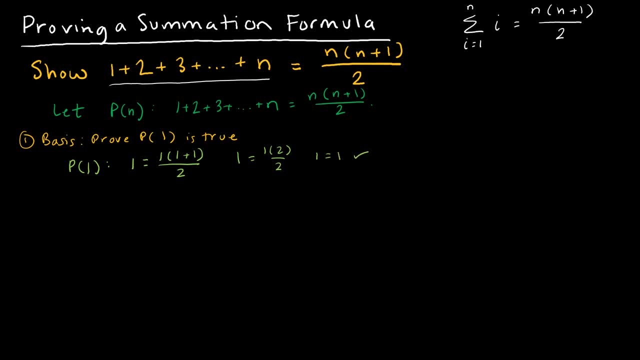 And so I get 1 equals 1, which is true. So I've proved the basis step. So that should always be a super duper easy step, because the first step, the basis step, is always going to be 1.. It's always just math. 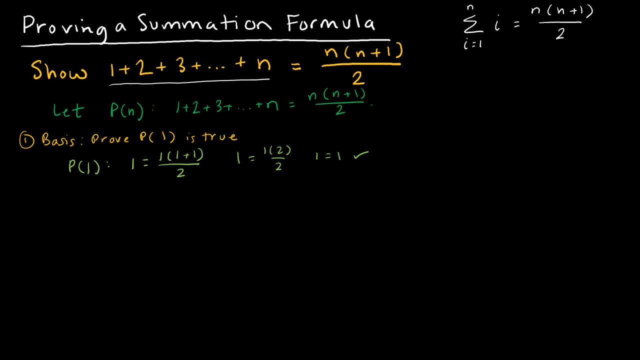 It's just plugging something in, So you don't have to prove anything. You're just plugging in something and verifying that it's true. Now the next step is where things get tricky. That is the inductive step. And remember: the inductive step says: assume that P of K is true. 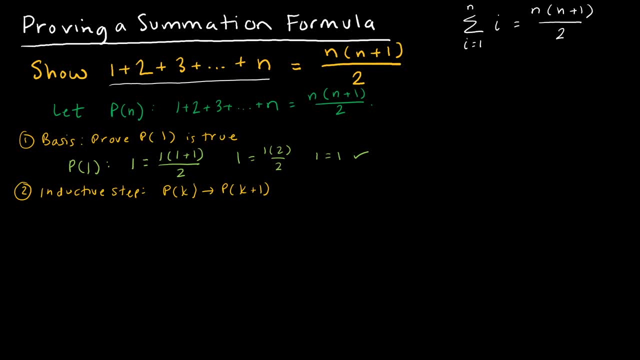 Prove that it implies P of K plus 1.. So there are two parts. So, in regards to this, I'm going to start by writing the inductive hypothesis. Yes, you always have to write that The inductive hypothesis is going to be exactly what P of N was. 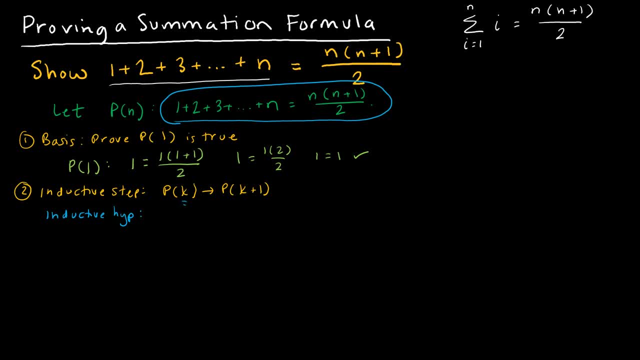 except we're going to plug K in instead, So it's super duper easy. So the inductive hypothesis is that 1 plus 2 plus 3, all the way through K is equal. So it's going to be equal to K times K plus 1 divided by 2.. 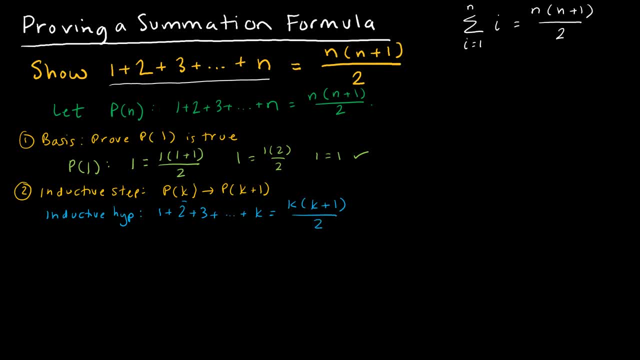 So I'm assuming P of K is true. Now this is the part that I said not all instructors show, But for me this is a really important step because this is my roadmap. This tells me what am I trying to get to. 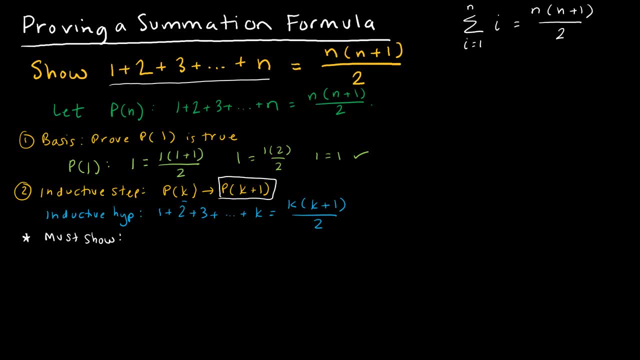 So I have to show: P of K plus 1 is true. So let's rewrite the inductive hypothesis as P of K plus 1.. So I have to show 1 plus 2.. 2 plus 3, all the way through: plus K plus K plus 1,. 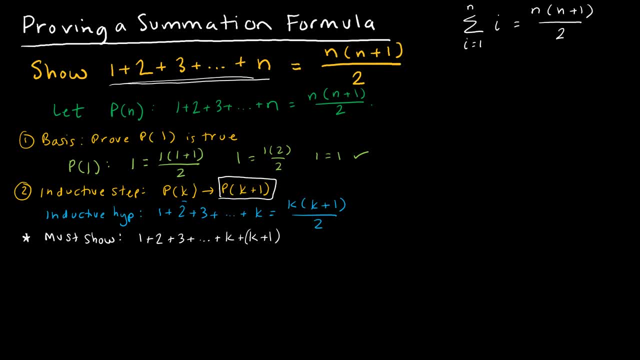 which would be my next term in the sequence- is equal to: And then again K. I have to add 1 because I'm doing K plus 1.. So this is K plus 1.. And then this was K plus 1.. 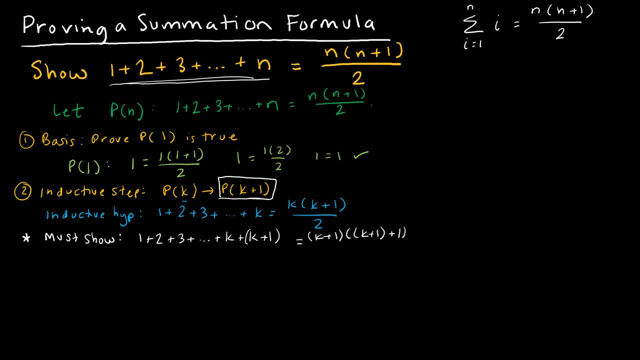 But I have to do K plus 1 plus 1 all divided by 2, which of course means that I'm showing that K plus 1 and this would be K plus 2 over 2.. So this is where I'm trying to get to. 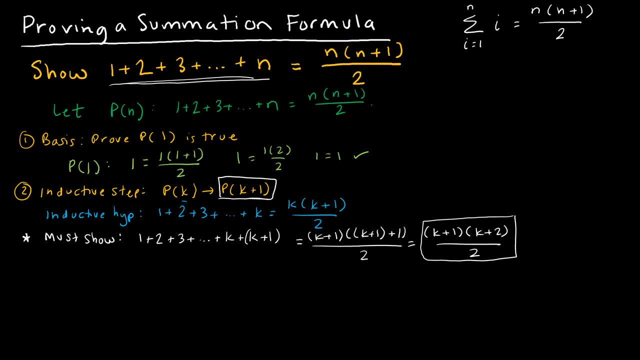 And again, that's why this step is important to me, because it gives me my roadmap. Where am I trying to end up? So now I'm going to start the induction part of this proof. I start with the inductive hypothesis 1 plus 2.. 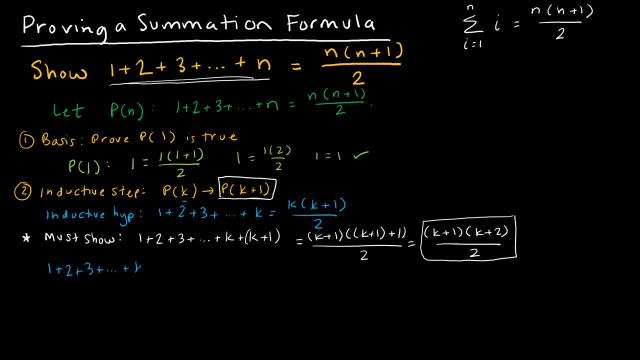 Plus 3.. Plus all the way through K, And remember I'm trying to show that this is true. So I'm going to then add K plus 1 to this side And then on the right side I have K times K plus 1 over 2.. 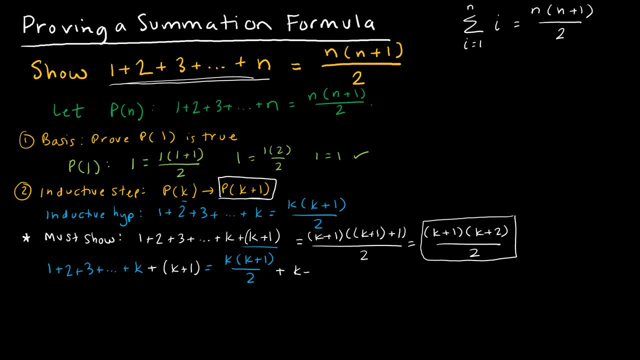 And whatever I did to the left side of an equation, I have to do to the right side of an equation, So that's my first step- is I'm adding K plus 1.. I'm adding K plus 1 to each side, So, as we can see, the left side here is exactly what I wanted. 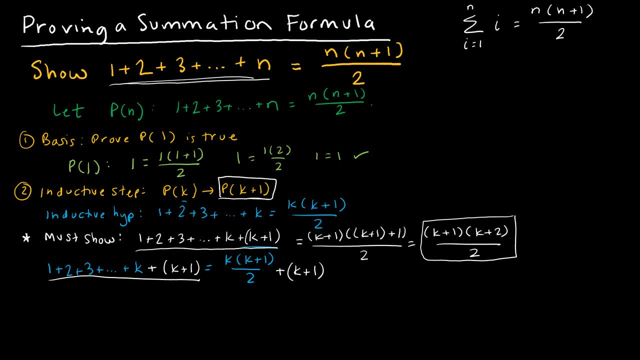 When I said this is what I must show. I have exactly what I must show. The right side, however, is not So. on the right side, that's where I'm going to do all of my work, So let's see what we can do here. 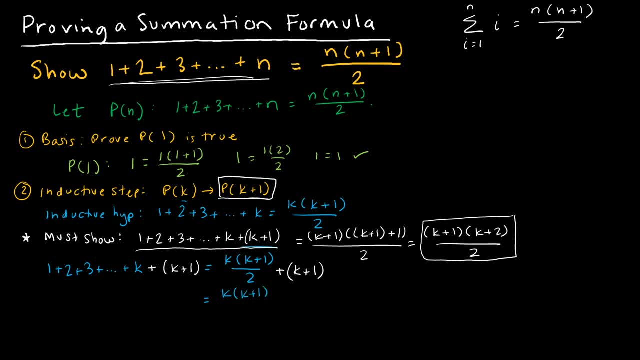 This is K times K plus 1 over 2.. And I want to add this to it. So I'm just going to add this to it And I'm going to multiply by 2 on top and on bottom. So plus 2 times K, plus 1 over 2.. 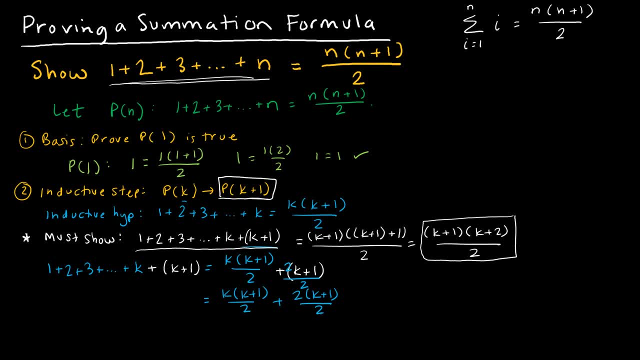 And the reason I'm going to do that is so then of course I can write it as a common sorry, write it as a fraction with a common denominator. So I could, of course, foil, I'm sorry, distribute the K, K squared plus K. 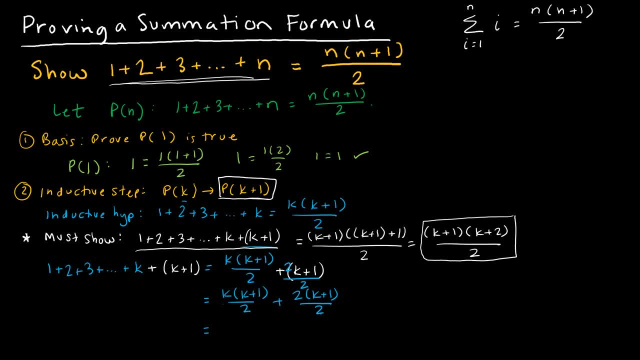 and then distribute the 2.. But what I know is essentially, this is one big fraction now with a plus in between and a denominator of 2. So what I have is factoring by grouping, where one of my factors is K plus 1. 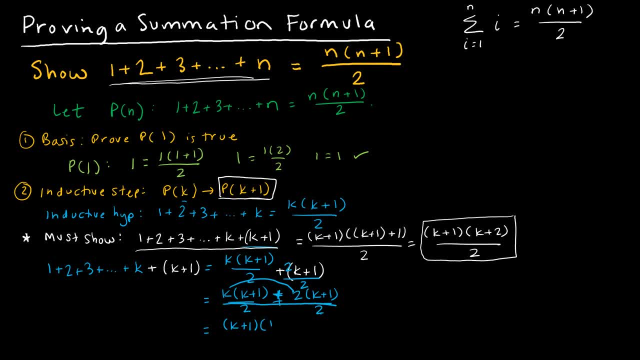 and the other factor is K plus 2, because that was their common factor. Both K and 2 have a common factor of K plus 1.. So this is my simplified solution. Now, did I do what I wanted to do? Yes, I did. 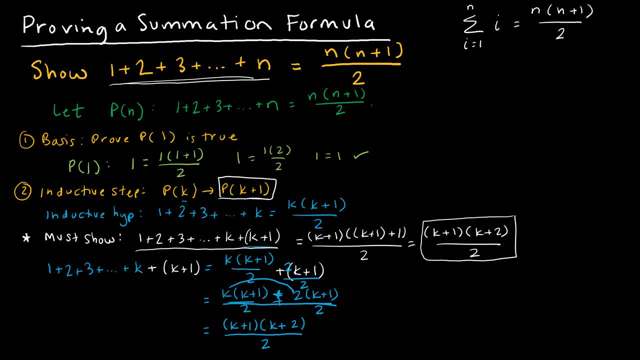 I've proved that by adding K plus 1 to each side, I did end up where I wanted to end up. So I'm done with my proof. So quite often at the end of the proof you'll see people then summarize: because this is true and this is true. 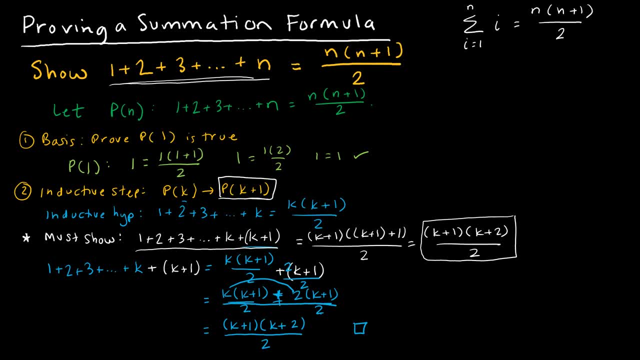 Then I've shown that this is true, And I've already done that by giving you this, my must show. So what I've done is I've now shown. so, therefore, P of n is true for all n that are positive integers. 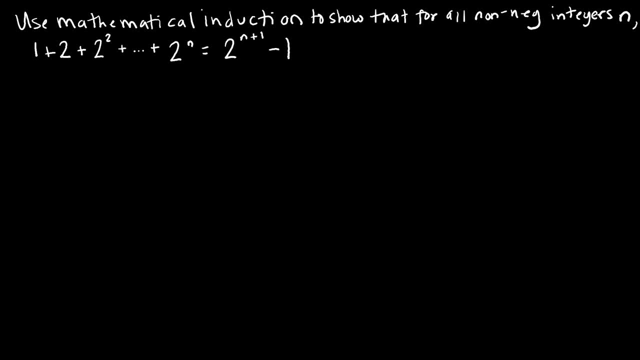 Let's do another proof, using induction. In this case, we want to show that for all non-negative integers, n. 1 plus 2 plus 2, squared all the way up through 2 to the n, is equal to 2 to the n plus 1 minus 1.. 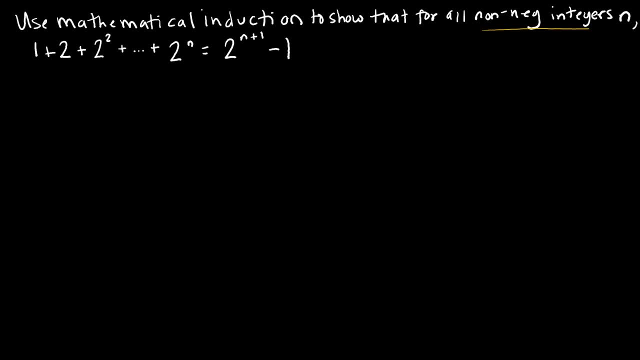 So one thing I want to point out is that we're dealing with all non-negative integers, So notice they didn't say positive integers, which means we're starting at 0,, 1,, 2,, 3,, et cetera. 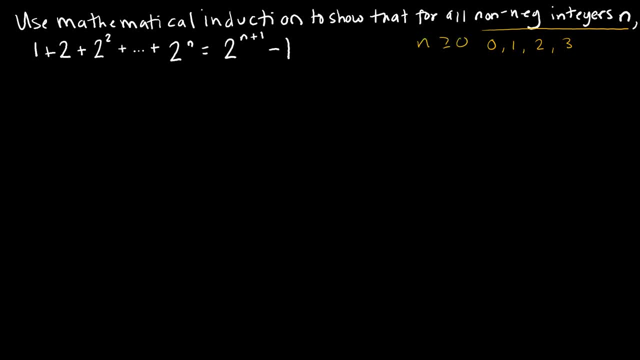 So n is greater than or equal to 0. That's going to come into play when we do our basis step. Before we do that basis step, let's take a look at what we're trying to show. So this is obviously 2 to the 0,. 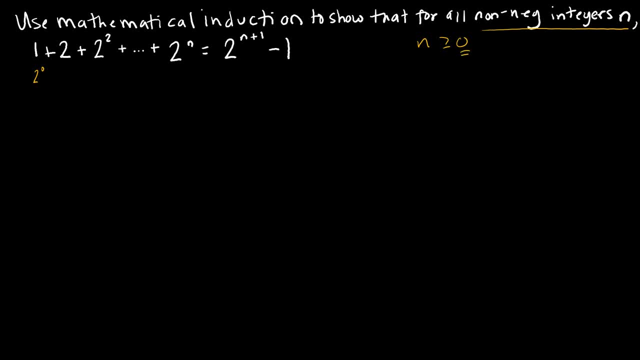 which makes sense, because we just talked about the fact we're starting at 0.. This is 2 to the 1st and this is 2 to the 2nd. So we can see that in fact, we were correct in saying n is greater than or equal to 0.. 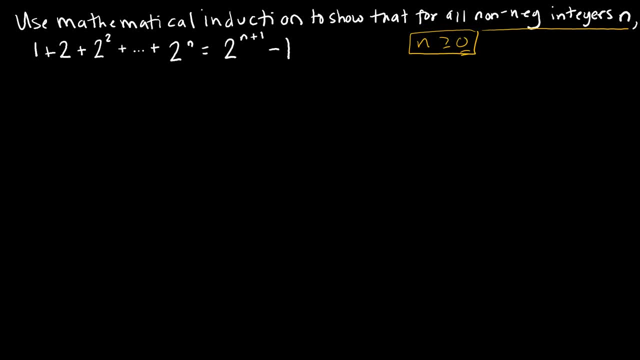 So now remember, our first step last time was that we have to specify what is P of n. So we're going to let P of n represent P of n, P of n, P of n. we're going to let P of n represent that 1 plus 2,. 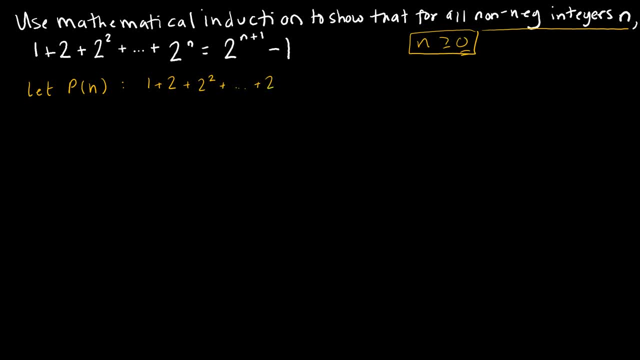 plus 2, squared all the way up through 2 to the n, is equal to 2 to the n, plus 1, minus 1.. Then we're going to start with our basis step, And remember our basis step is to prove P of 1.. 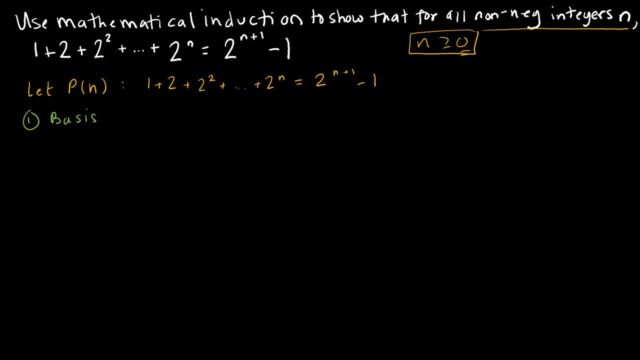 Now be careful, Remember. the basis step just says: Hey, prove the very first element. and we just talked about the first element being 0. So I need to show that P of 0, that P of 0, 0 is true. So p of 0 would be: 2 to the 0 is equal to 2 to the 0 plus 1 minus 1.. While 2 to the 0 is. 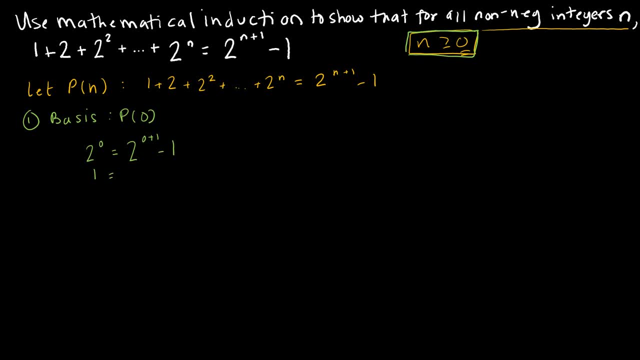 1,. 2 to the 0 plus 1 is 2 to the first, which is 2 minus 1 is 1.. So I've shown the basis step to be true. Now let's look at our inductive step And recall. our inductive step says: assume pk. 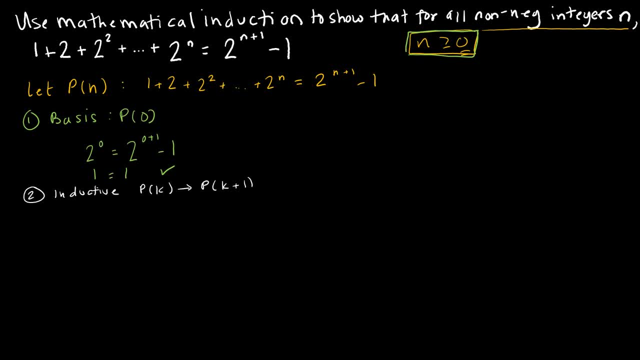 show that implies p of k plus 1.. So we start by writing our inductive hypothesis, which is exactly what my p of n statement is, with k's instead, every single time. So 1 plus 2 plus 2, squared all the way up through 2 to the k, is equal to 2 to the k plus 1 minus 1.. And then 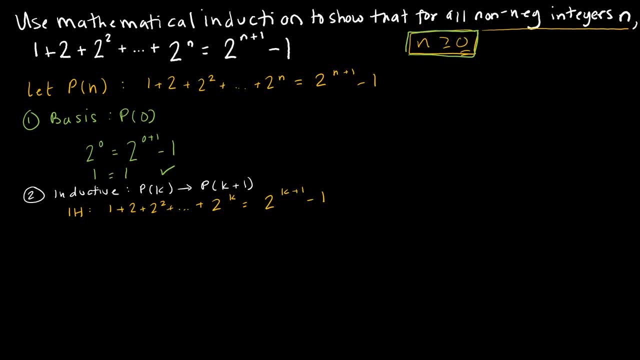 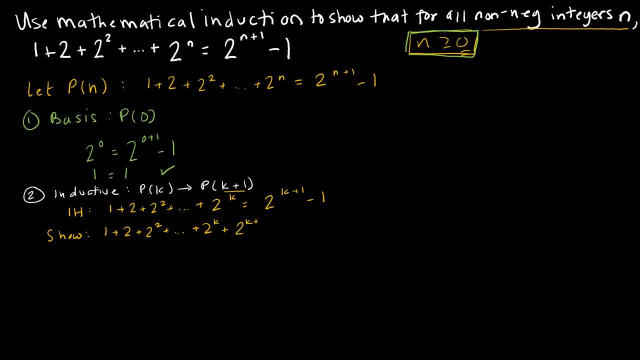 Plus 2 to the k plus 1 is equal to 2 to the k plus 1 plus 1 minus 1, which, of course, is 2 to the k plus 2 minus 1.. So this is what I'm trying to get to, And now let's go ahead and go for it. So. 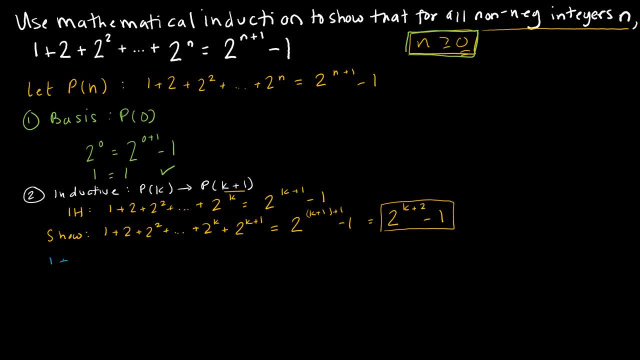 I'm going to start with my inductive hypothesis: 1 plus 2 plus 2 squared, 2 squared all the way up to 2 to the k. and what am I going to add to that? I'm going to add 2 to the k plus 1, and again, why did I add 2 to the k plus 1? Because I want the left side. 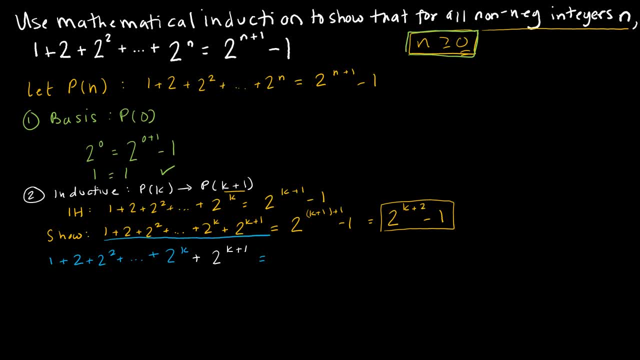 to be exactly what I'm trying to show On the right side. again, I'm using the inductive hypothesis 2 to the k plus 1 minus 1, and to be mathematically correct, I have to then add exactly what I added to the left side: 2 to the k plus 1.. Now, what am I going to do? 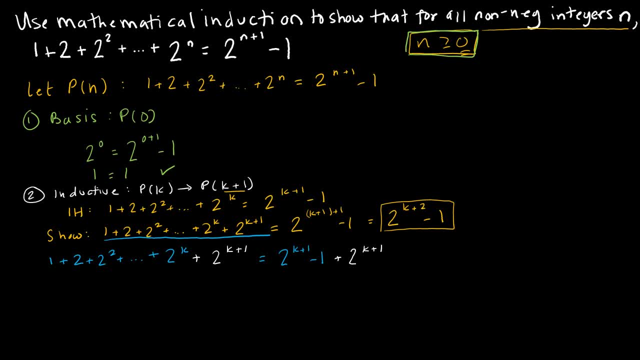 Well, the left side's exactly as I want it, so I'm going to leave it just like that. The right side. what I have is obviously again: this is where the algebra comes in. I've got 2 to the k plus 1,. 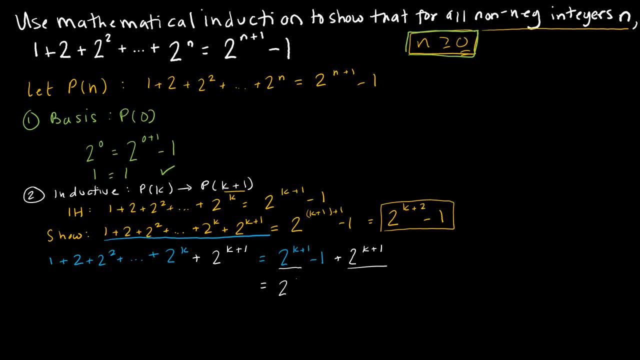 and I've got another 2 to the k plus 1, so I actually have 2: 2 to the k plus 1's minus 1.. Well, what's 2? 2 to the k plus 1?? Remember if you have two values with the same base. 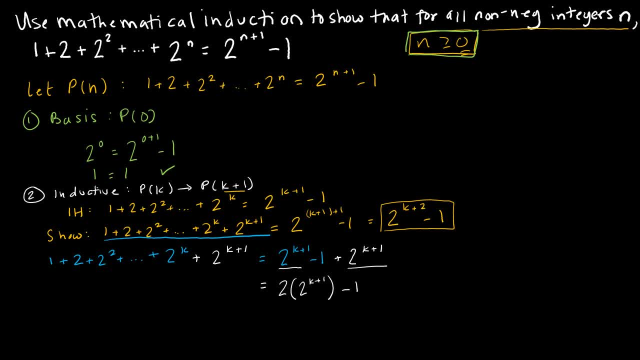 that you're multiplying. you can add the exponents together, Like if I had 3 squared times 3 to the 4th, that would be the same as 3 to the 6th. I can add the 2 plus the 4.. 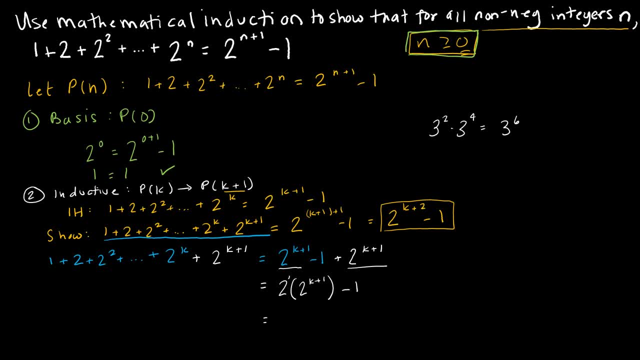 That's all I'm going to do. So 2 to the 1st and 2 to the k plus 1 would be 2 to the k plus 2, and I still have my minus 1.. And so did I do what I set out to do in the beginning. Yes, I did again. 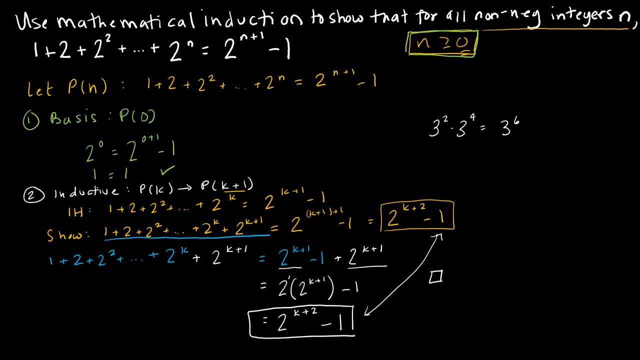 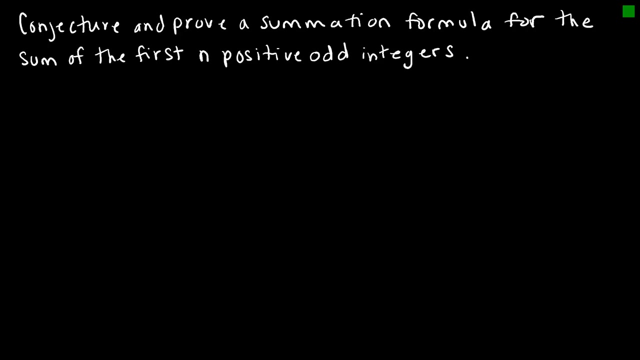 because these two things match up. Therefore, I'm done and I can say that p of n is true for all n greater than or equal to 0, where n, obviously is an integer. So let's take a look at one that's a little bit harder. And this one's harder not because it's 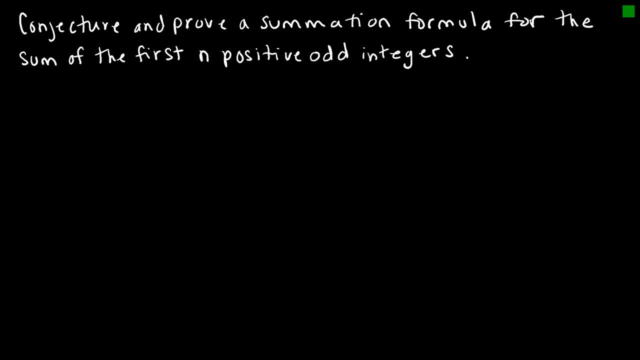 a harder proof, but because I haven't given you what to prove, And so if I don't give you what to prove, it's up to you to conjecture what it is that I should be proving and then prove it. So it's really two parts. 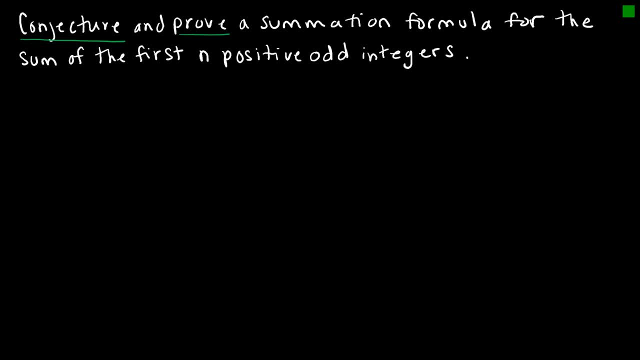 And so this is talking about the sum of the first n positive odd integers. So best idea here is to just start plugging and chugging and seeing if we can see a pattern. So we're going to look at it: for n equals 1, for n equals 2, for n equals 3, n equals 4.. And can we then justify that? for n? 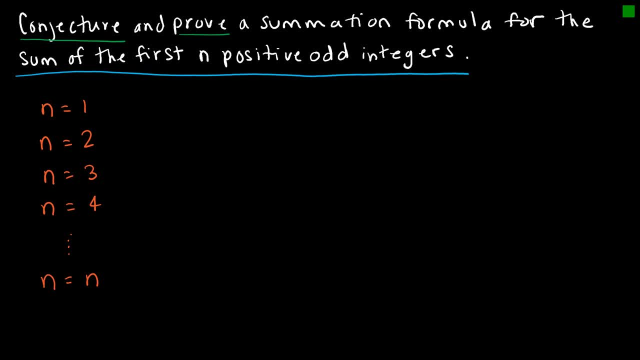 equals n, So for 1,. obviously that just stays the same. So we're going to look at it: for n equals 2,, for n equals 3,, n equals 4, and can we then justify that? for n equals n, So for 1,. obviously that just. 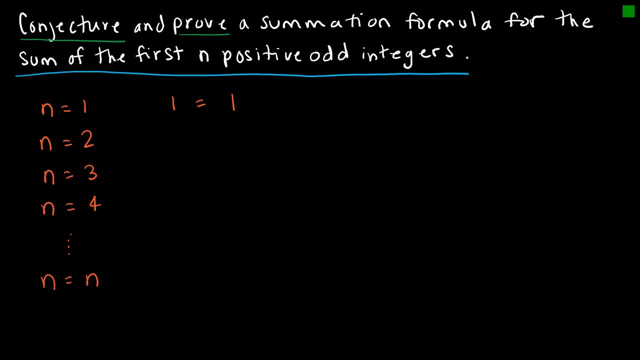 means the sum of 1, which is 1.. For 2,, that means the first two positive odd integers, so that's 1 plus 3, and 1 plus 3 is 4.. For n equals 3, that means three integers: 1 plus 3 plus 5,, which is. 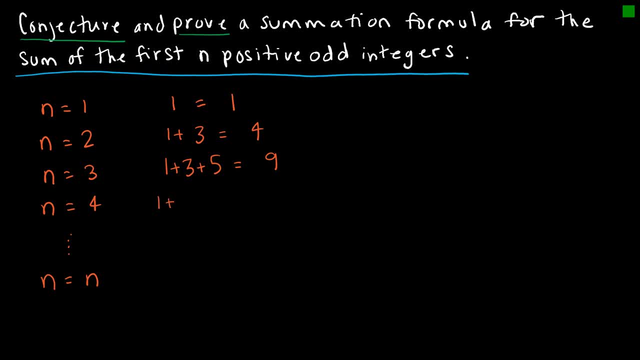 9.. For 4, it's 1 plus 3 plus 5 plus 7, which is 16.. And what I'm looking at is: is there a pattern? and this appears to be 1 squared and 4 is 2 squared and 3 is 3 squared, or 9,? excuse me, 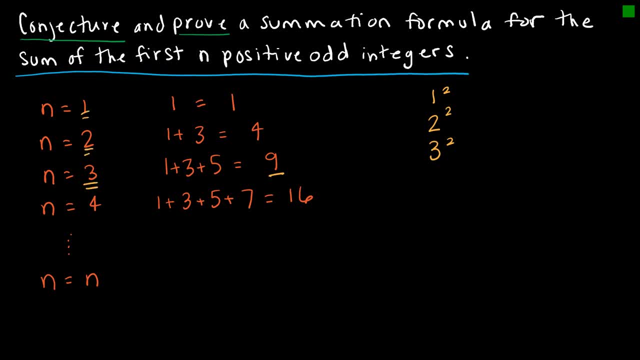 is 3 squared. I was looking at this 3, and, as we can see, what I'm ending up with down here seems to be n squared, which is fantastic, because now I have an idea of what that sum will be. What I also need to look at is: how would I write this? 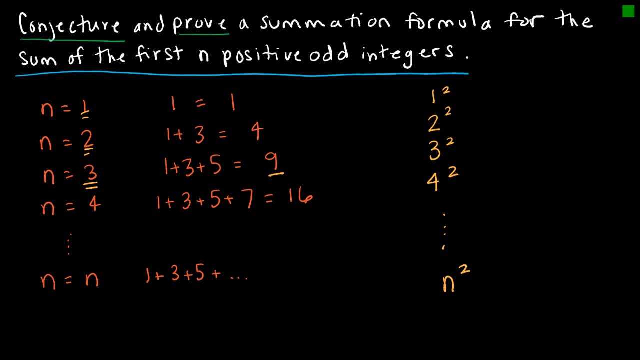 in terms of n on this side, Because- remember, I want this to be my statement- that the sum of all of these values is equal to n squared, and so I have to look at what would I do with n to find the next integer. So to get 3 from 4,, I'm sorry, to get 3 from 2,. to get 5 from 3,. 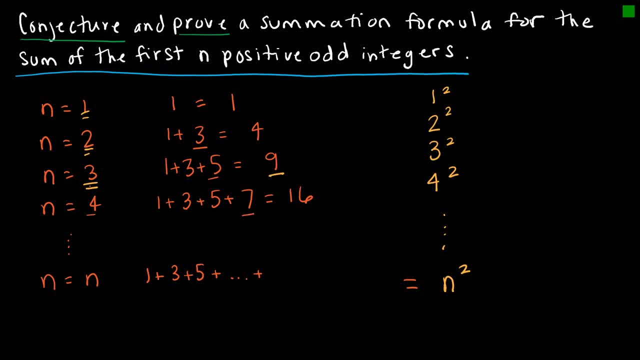 to get 7 from 4, to get 5 from 3, to get 7 from 4, to get 7 from 4, to get 7 from 4, to get 7 from the 4,, being that's the next integer that I'm adding, means that I'm actually taking 2 times n. 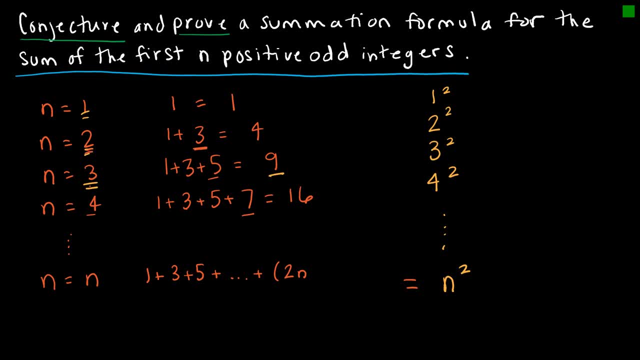 so 2 times 2 would be 4, minus 1 to get 3.. 2 times 3 is 6, minus 1 to get 5.. 2 times 4 is 8, minus 1 to get 7.. So that is my formula. So obviously that part wasn't super easy. 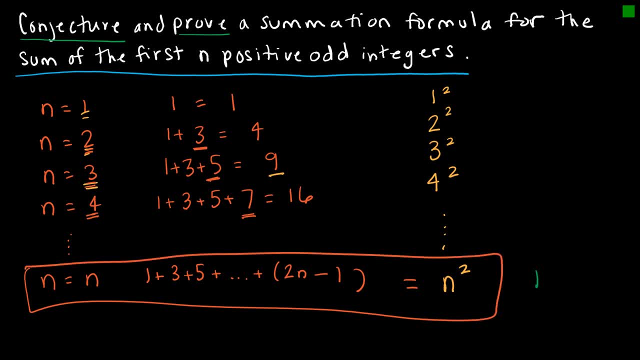 This is going to end up being when I do this on the next page. this is going to end up being when I do this on the next page. my statement p of n is that 1 plus 3 plus 5 plus dot, dot, dot plus 2n minus 1 is equal to n squared. 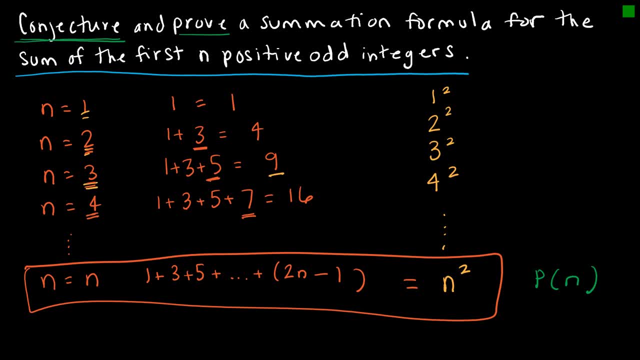 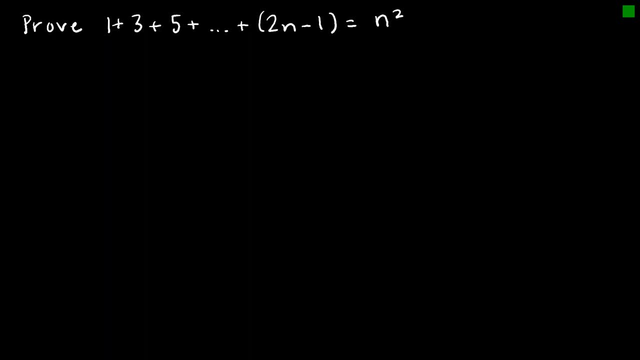 So now that I have come up with- I've conjectured- my summation formula, now I want to actually prove it. So now that I've done the work to come up with the formula that I think is right, I actually have to prove it. And so, again, I'm going to start by just explicitly saying: 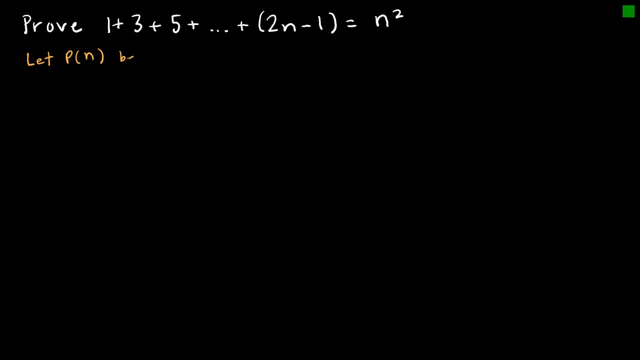 that p of n be the proposition that 1 plus 3 plus 5, etc, etc, all the way up to 2n minus 1 is equal to n squared. So I'm just explicitly saying that is true And then I need to show my basis step And remember my basis step. 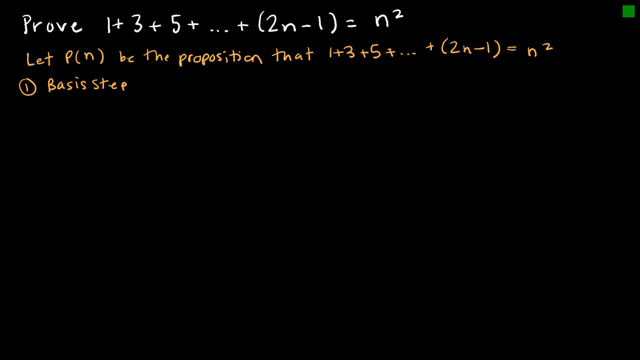 just is n squared. So I'm just explicitly saying that is true. And then I need to show my basis step, looking at the lowest value. And so, if we're looking at this, we really started with n being a positive integer And so that my basis step would be the lowest positive integer. So I have to prove. 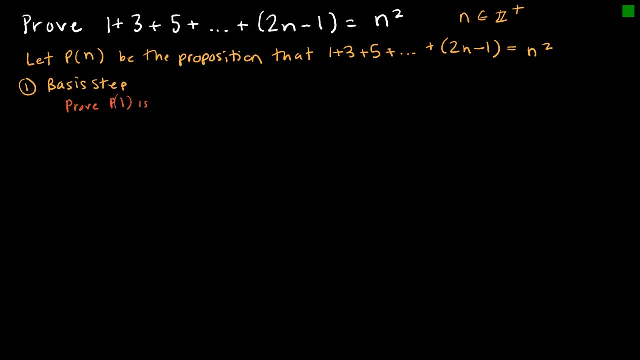 that p of 1 is true, And what I can do then is say: well, that would be: 1 equals 1 squared, And is that true? Yes, 1 equals 1.. Therefore, the basis step is proven. We'll do it that way. 1. 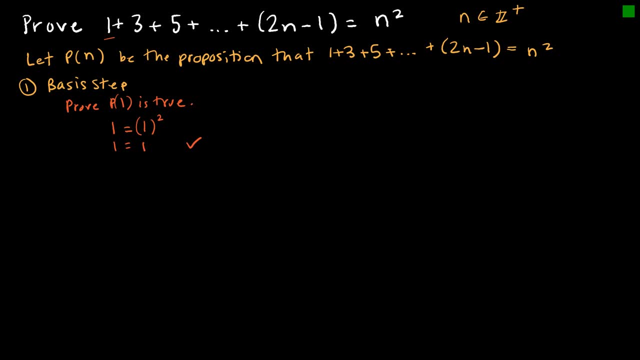 equals 1.. The next step is the induction step, or the inductive step, And remember that says: assume p of k is true, show p of k plus 1 is true. And again I like to write it out explicitly And: 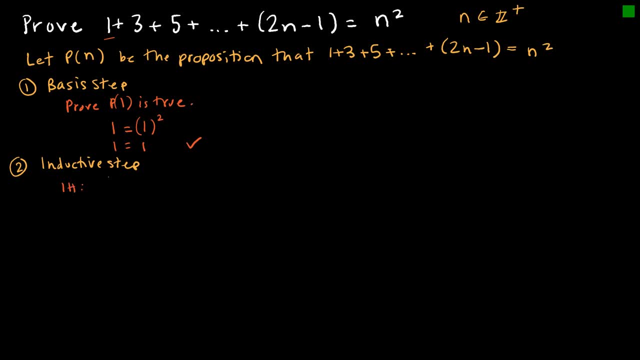 you have to write the inductive hypothesis. The inductive hypothesis is that 1 plus 3 plus 5, etc. etc. all the way up to 2k minus 1 is equal to k squared, Because again we're looking at p of k being true. Then I want to show, and again I like to: 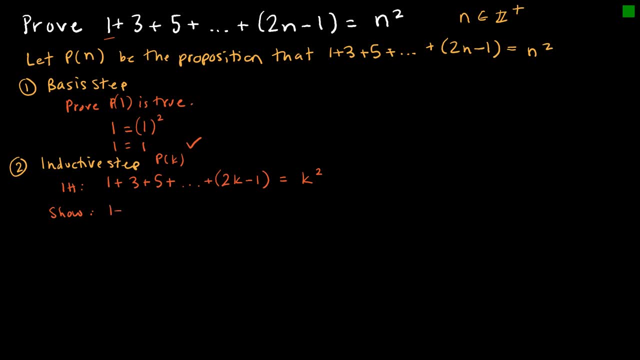 write this step so I know where I'm headed. I want to show that if I continued this, if I continued this, I would have 2k plus 1 squared, And I added the next integer, And so the next integer would be 2 more than 2k minus 1, which would be 2k plus 1.. I want to show that if I add. 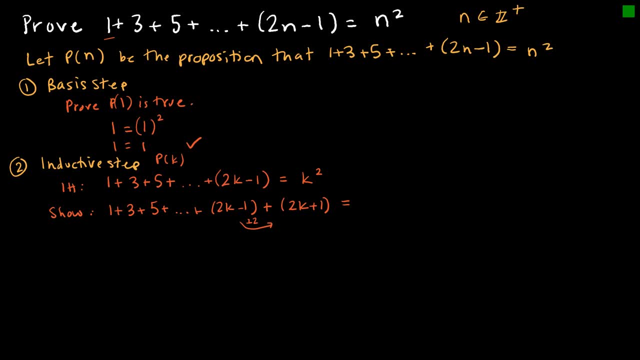 that to the left side, then the right side will become k plus 1 squared. So that is what I'm trying to get to is saying I'm going to add the next odd integer And I should end up with k plus 1 quantity squared as my solution. So now let's go about doing this. I have 1 plus 3 plus 5 plus. 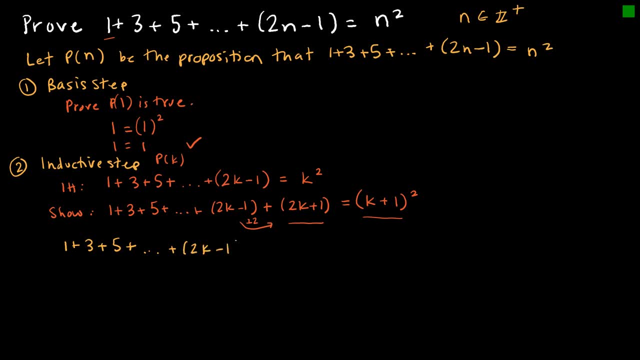 blah, blah blah, plus 2k minus 1,, which I know is true, And that is equal to k squared, which I know is true. And I also know that if I add something equal to each side, then the equation still holds. So I'm going to add 2k plus 1 to each side of the equation. 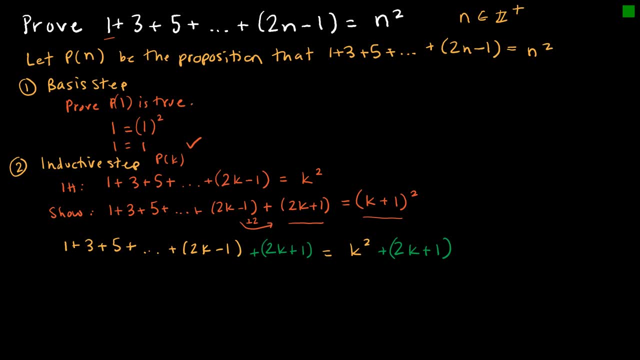 So I haven't broken any mathematical laws. I've added something equal to each side. Now, on the left side, this is exactly what I wanted. I have the same series or progression that I had before, And all I've done is now add 2k plus 1,, which is what I wanted to get to. 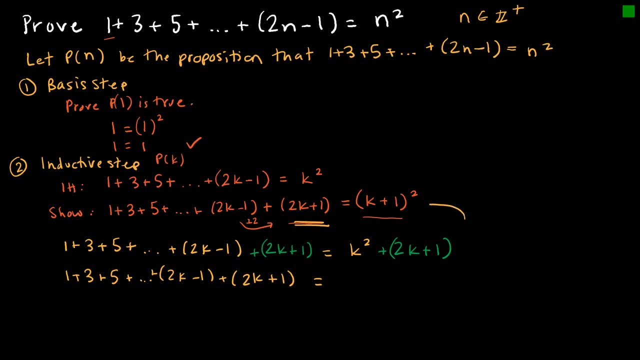 And on the right side, I'm trying to see if that is in fact equal to k plus 1, quantity squared, And so what I'm looking at is I have three terms: k squared plus 2k plus 1.. And it looks like I can. 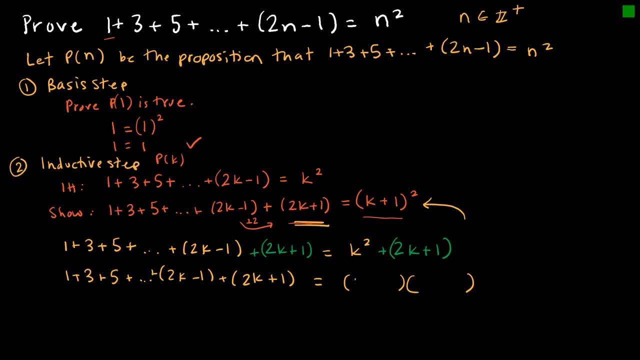 factor those, And if I factor, I'm looking for numbers that multiply to 1, that add to 2, which is 1 and 1.. So this would actually be k plus 1, k plus 1.. And of course that means